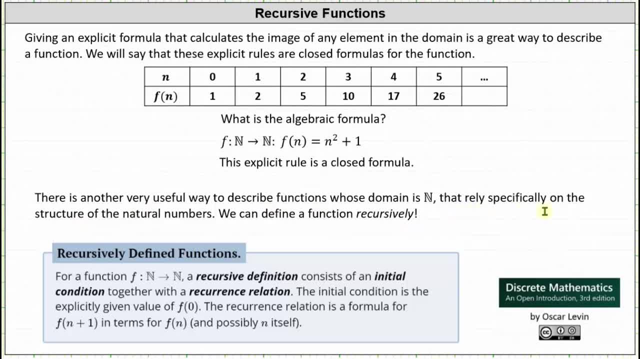 functions whose domain is the set of natural numbers that rely specifically on the structure of the natural formula. So in this case the closed formula is: f of n equals n squared plus one. We can define a function recursively For a function f which maps the set of natural numbers. 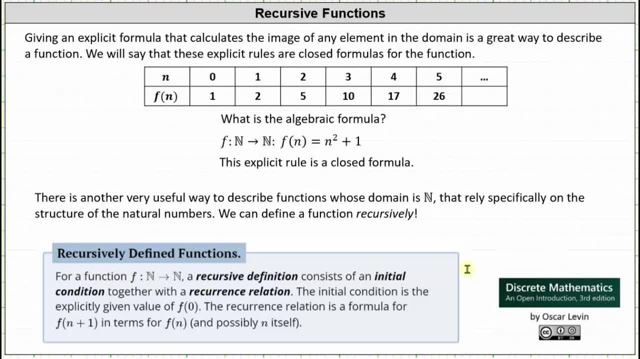 to the set of natural numbers. a recursive definition consists of an initial condition together with a recurrence relation. The initial condition is explicitly given as the value of f of zero, and the recurrence relation is a formula for f of n plus one in terms of f of n, which. 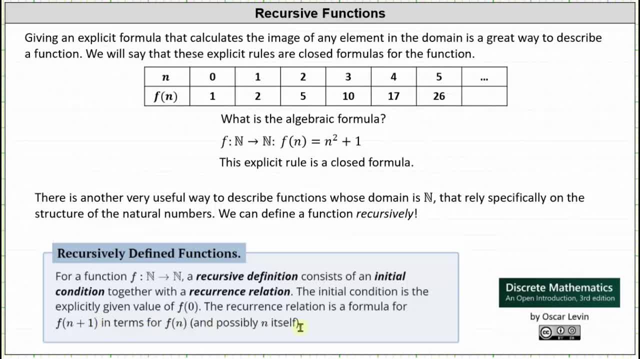 means to determine f of n plus one. we do need f of n where f of n equals n squared plus one, where for an explicit formula or a closed formula we only need the value of n or the input. Let's see if we can determine the recursive function for the same function shown above. 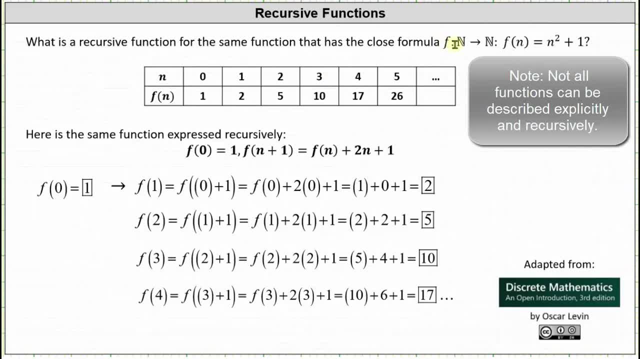 Again, we already know we can describe the function below as the function that maps the set of natural numbers to the set of natural numbers, such that f of n is equal to n squared plus one. but we can also describe the same function using a recursive function. 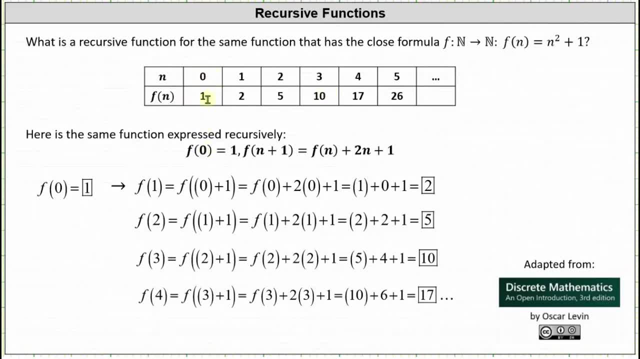 where to begin. we have: f of zero is equal to one from the first column in the table and the recurrence relation is: f of n plus one is equal to f of n plus two, n plus one, which means to find f of n plus one. we take the previous function value. 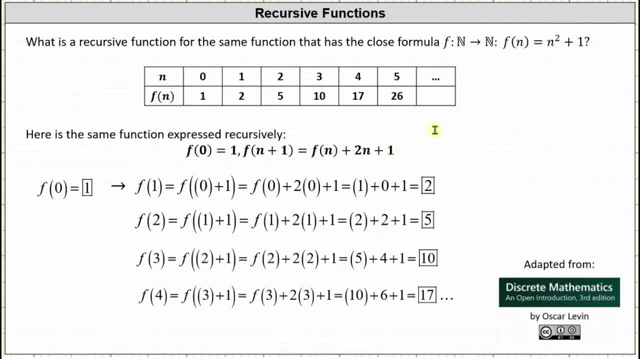 and add two times n plus one. So, looking at our work below, we know f of zero is equal to one, because that's given to determine f of one. notice: n is equal to zero, since f of zero plus one is equal to f of one, which indicates that f of one is equal to f of. 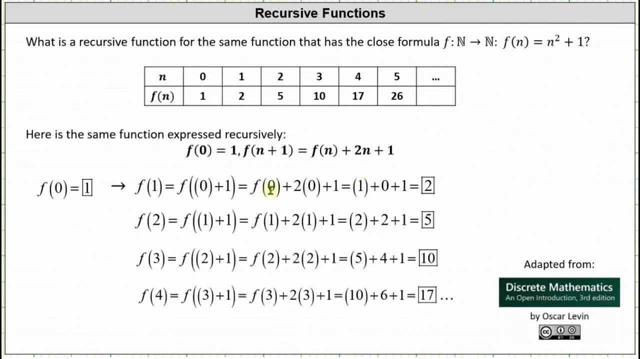 0 plus 2 times 0 plus 1.. And we know f of 0 is equal to 1, indicating f of 1 is equal to 1 plus 0 plus 1, which is equal to 2.. Now that we know f of 1, we can determine f of 2.. Notice for f of 2,. 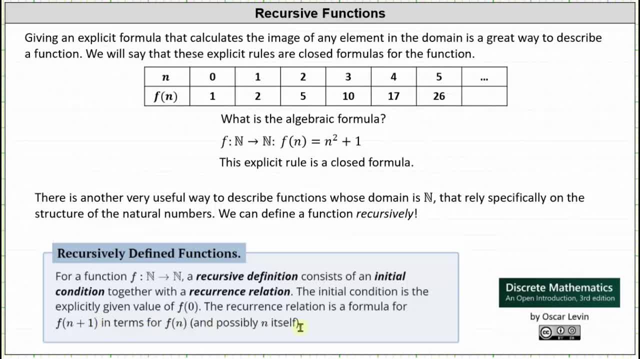 means to determine f of n plus one. we do need f of n where f of n equals n squared plus one, where for an explicit formula or a closed formula we only need the value of n or the input. Let's see if we can determine the recursive function for the same function shown above. 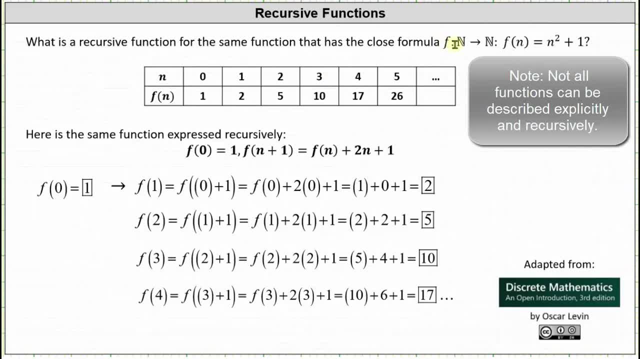 Again, we already know we can describe the function below as the function that maps the set of natural numbers to the set of natural numbers, such that f of n is equal to n squared plus one. but we can also describe the same function using a recursive function. 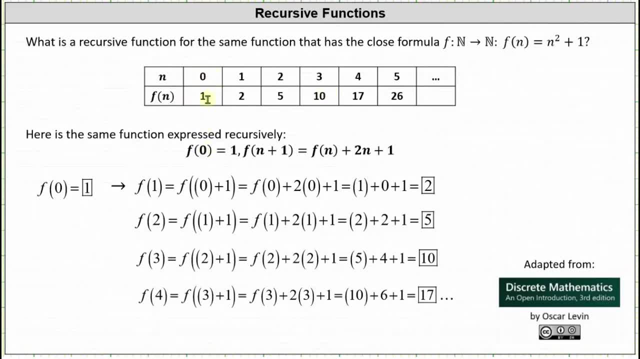 where to begin. we have: f of zero is equal to one from the first column in the table and the recurrence relation is: f of n plus one is equal to f of n plus two, n plus one, which means to find f of n plus one. we take the previous function value. 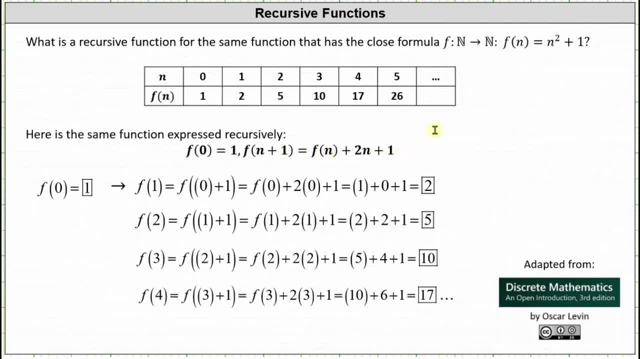 and add two times n plus one. So looking at our work below, we know f of zero is equal to one, because that's given To determine f of one. notice: n is equal to zero, since f of zero plus one is equal to f of one. 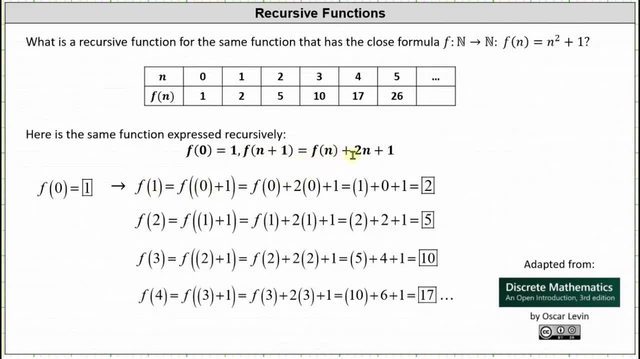 which indicates that f of one is equal to f of zero plus two times zero plus one. and we know f of zero is equal to one, indicating f of one is equal to one plus zero plus one which is equal to two. Now that we know f of one, we can determine f of two. 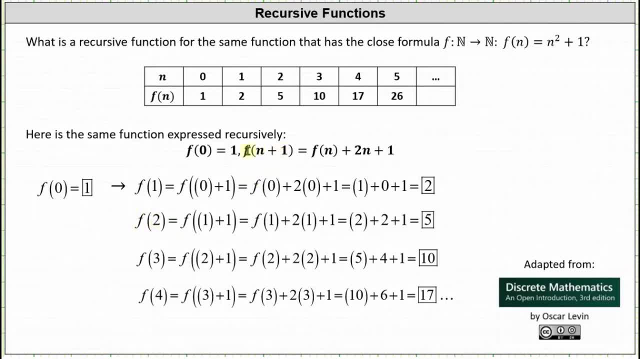 Notice for f of two, n is equal to one. giving us f of one plus one or f of two which is equal to f of one plus two, times one plus one, Again we know: f of one is equal to two, f of two is equal to two plus two plus one, which is equal to five. 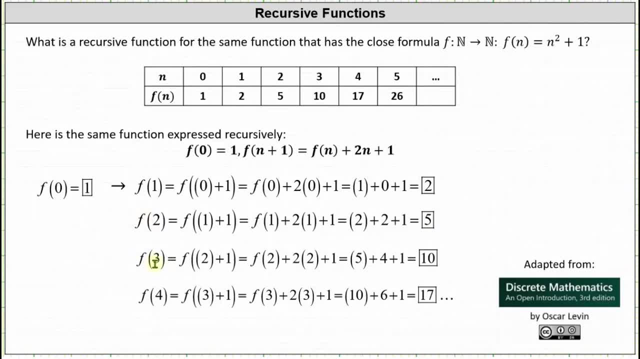 Now that we know f of two, we can determine f of three. To determine f of three, notice: n is equal to two, since two plus one is three. giving us f of three is equal to f of two plus two times two plus one. And again we know: f of two is five, f of three is equal to five. 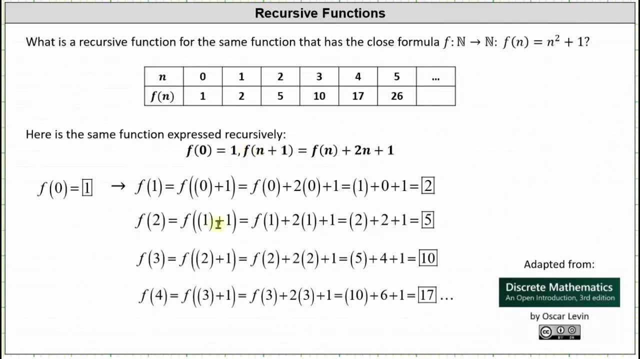 n is equal to 1, giving us f of 1 plus 1 or f of 2, which is equal to f of 1 plus 2 times 1 plus 1.. And again we know: f of 1 is equal to 2.. f of 2 is equal to 2 plus 2 plus 1, which is equal to 5.. 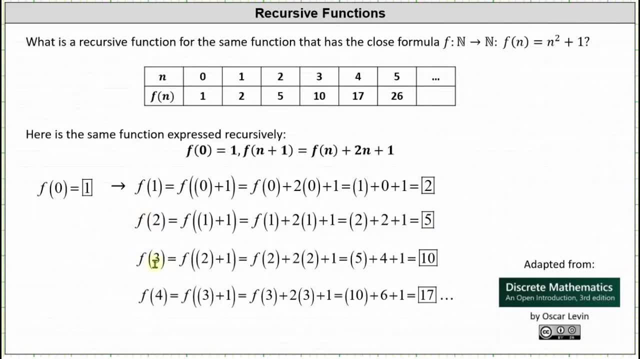 Now that we know f of 2, we can determine f of 3.. To determine f of 3, notice n is equal to 2, since 2 plus 1 is 3, giving us f of 3 is equal to f of 2 plus 2 times 2 plus 1.. 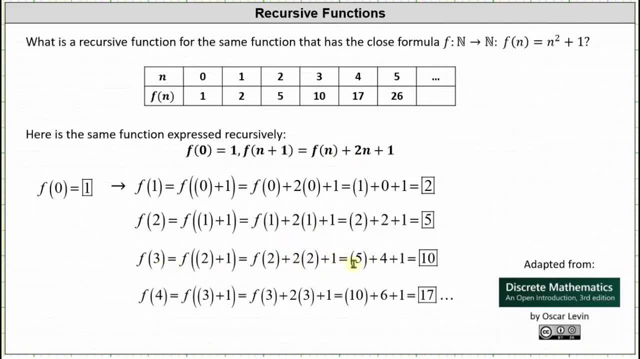 And again, we know: f of 2 is 5.. f of 3 is equal to 5 plus 4 plus 1, which equals 10.. Okay, now that we know f of 3, we can determine f of 4.. Notice: for f of 4, n is equal to 3,. 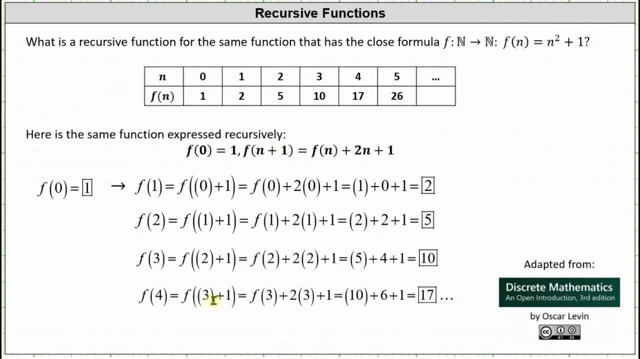 since 3 plus 1 is 4, giving us f of 4 is equal to f of 3 plus 2 times 3 plus 1.. f of 3 is 10, 2 times 3 is 6.. f of 4 is equal to 10 plus 6 plus 1,, which is equal to 17.. So notice the drawback. 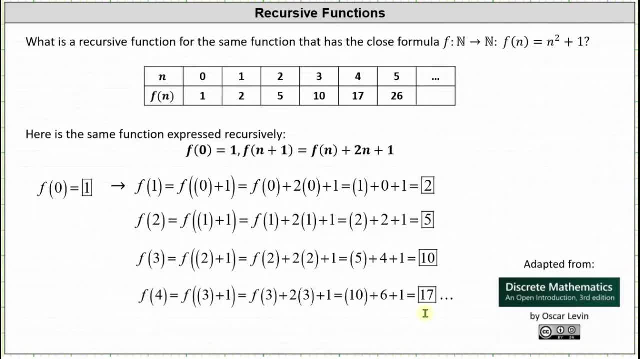 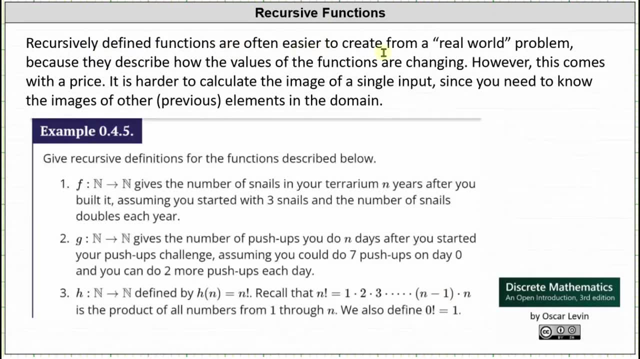 on recursive functions is that we do have to know previous function value or values to know that we know f of 3. determine the next function value. However, recursively defined functions are often easier to create from a real-world problem because they describe how the values of the functions are. 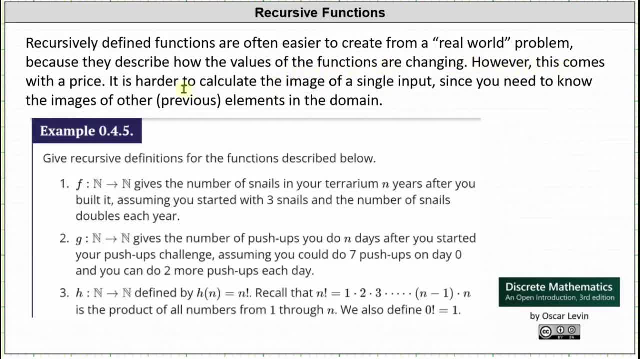 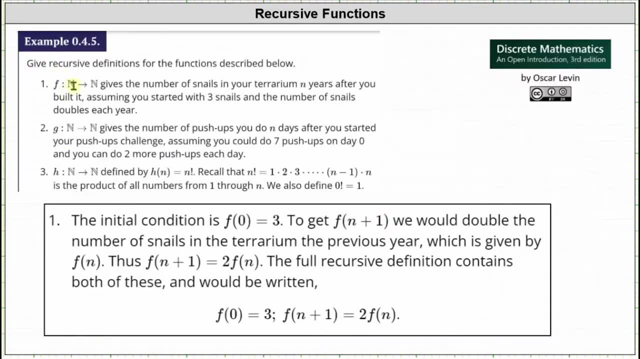 changing But, as I just mentioned, this comes with a price. It is harder to calculate the image of a single input, since we need to know the images of other previous elements in the domain. Let's look at the three examples below. Number one: we have the function f, which again maps the set of natural 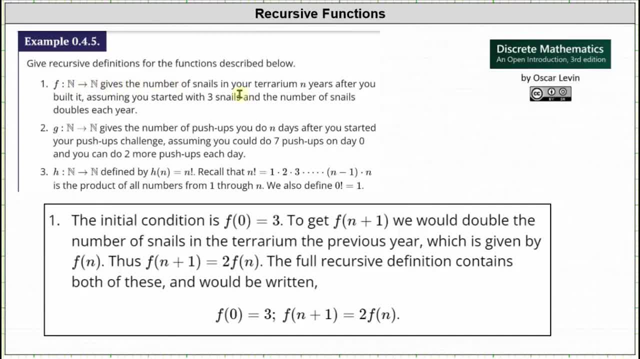 numbers to the set of natural numbers which gives the number of snails in your terrarium and years after you built it. assuming you started with three snails and the number of snails doubles each year, The initial condition is f of 0 equals 3,. since you start with three snails, To get f of 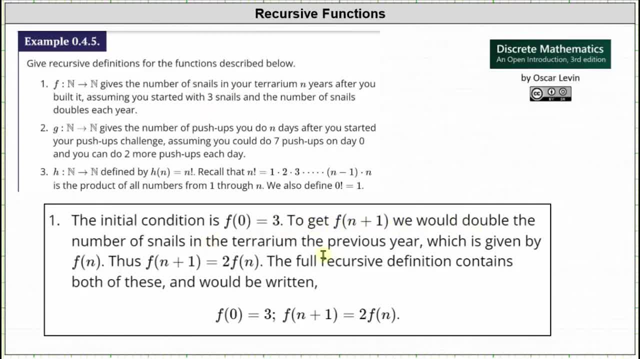 n plus 1, we would double the number of snails in the terrarium the previous year, which is given by f of n, which gives us f of n plus 1 is equal to 2 times f of n. The full recursive definition contains both the initial condition and the recurrence formula, or. 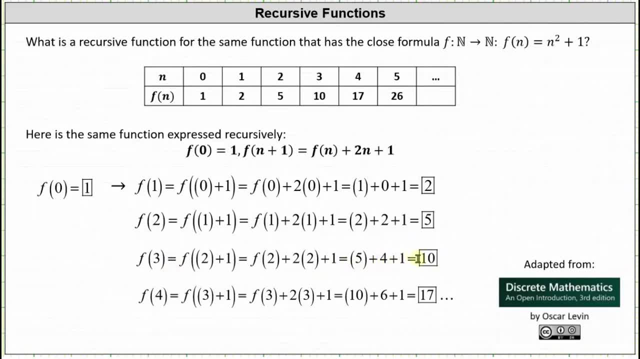 plus four plus one, which equals 10.. And now that we know f of three, we can determine f of four. If we know if one is equal to n plus one, it will also give us f of two. Notice for f of four. 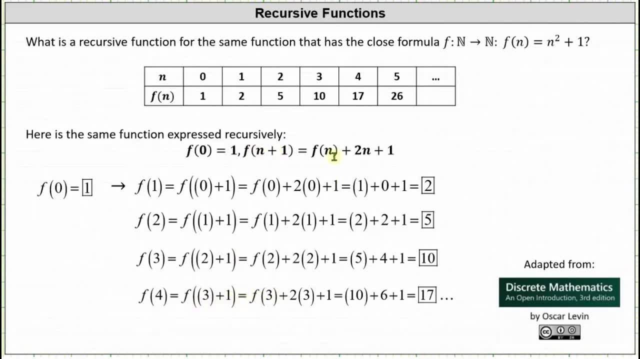 n is equal to three. since three plus one is four, giving us f of four is equal to f of three plus two times three plus one. f of three is ten. two times three is six. f of four is equal to 10 plus six plus one, which is equal to 17.. So notice the drawback. 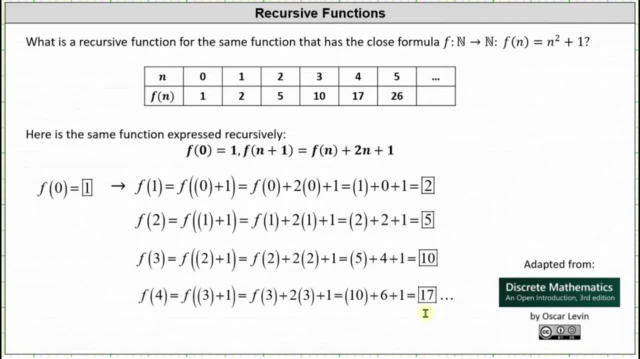 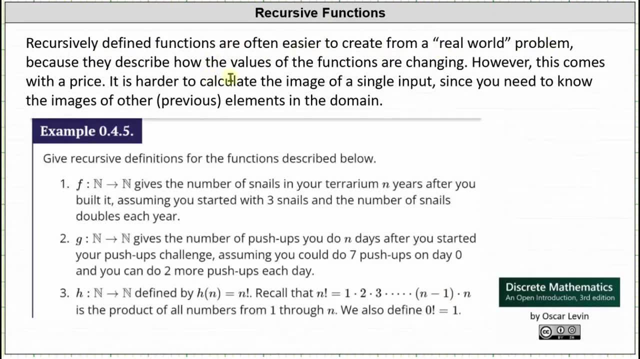 on recursive functions is that we do have to know previous function value or values to determine the next function value. Diversively defined functions are often easier to create from a real world problem because they describe how the values of the functions are changing. But, as I just mentioned, this comes with a price. 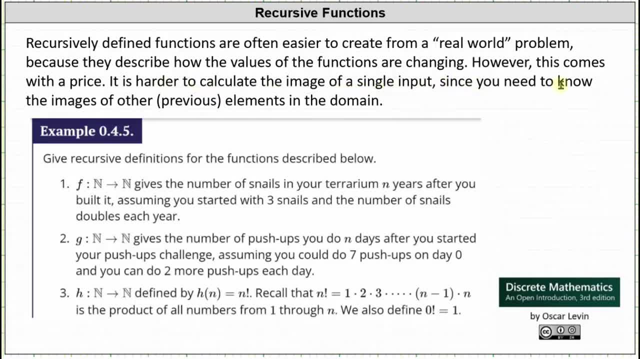 It is harder to calculate the image of a single input, since we need to know the images of other previous elements in the domain. Let's look at the three examples below. Number one: we have the function f, which again maps the set of natural numbers. 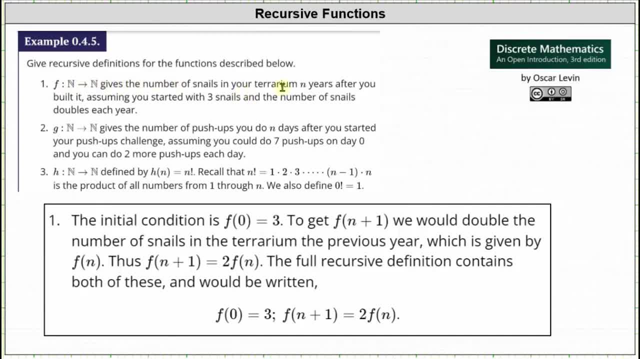 to the set of natural numbers which gives the number of snails in your terrarium and years after you built it. assuming you started with three snails and the number of snails doubles each year, The initial condition is f of zero equals three. 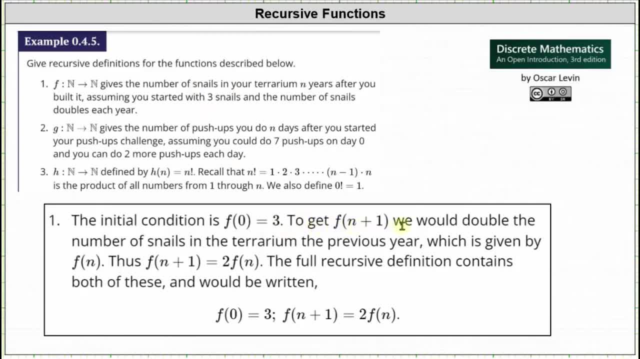 since you start with three snails, To get f of n plus one, we would double the number of snails in the terrarium the previous year, which is given by f of n, which gives us f of n plus one, is equal to two times f of n. 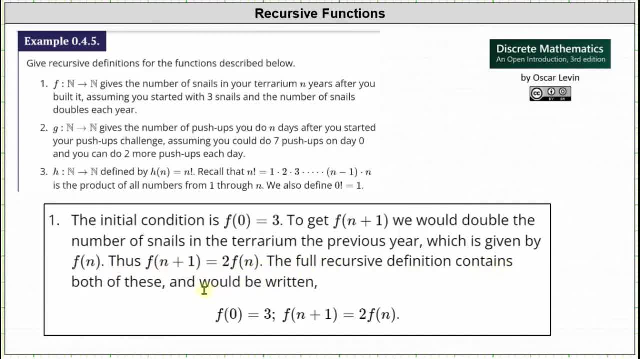 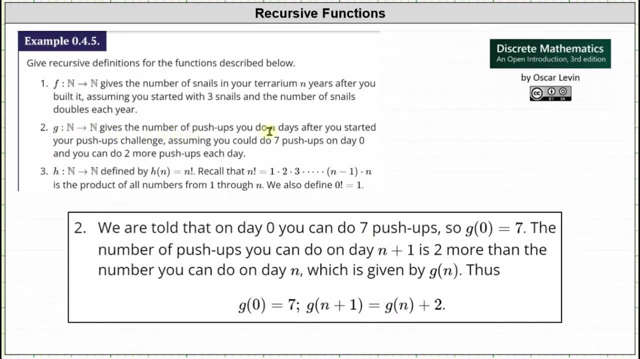 The full recursive definition contains both the initial condition and the recurrence formula or recurrence relation, given by: f of zero equals three and f of n plus one equals two times f of n. For number two we have the function g, which gives the number of pushups you can do. 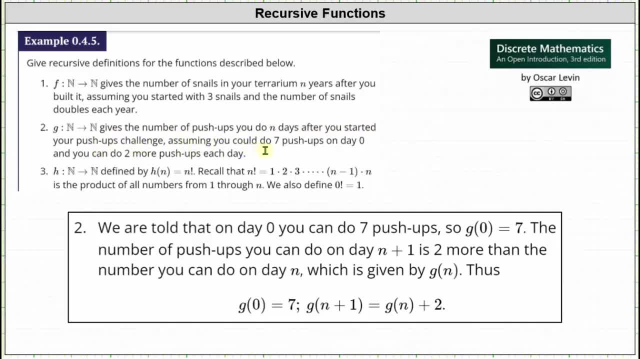 n days after you started your pushups challenge, assuming that you can do seven pushups on day zero and you can do two more pushups each day. So we are told that on day zero you can do seven pushups. That's right, seven pushups. 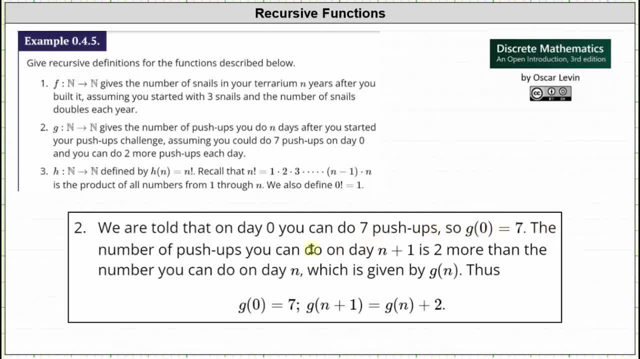 which indicates g of zero equals seven. The number of push-ups you can do on day n plus one is two more than the number of days you can do on day n, which is given by g of n, and therefore we have: g of zero equals seven, and g of n plus one is equal to g of n plus two. And then for number three, 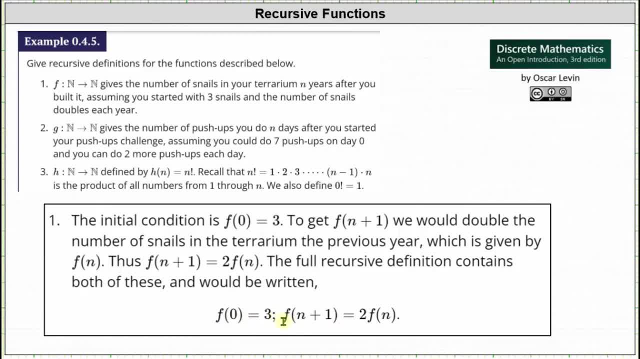 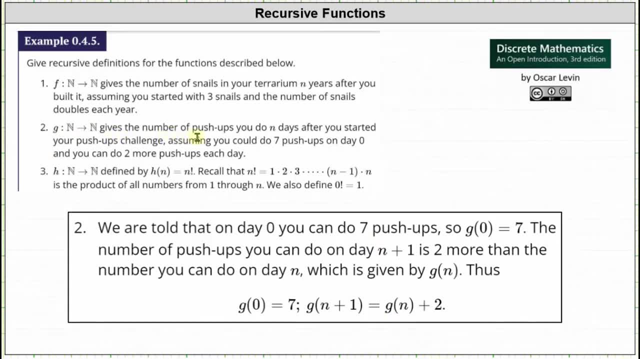 recurrence relation given by f of 0 equals 3 and f of n plus 1 equals 2 times f of n. For number two, we have the function g, which gives the number of push-ups you can do n days after you started your push-ups challenge, assuming that you can do seven push-ups on day 0.